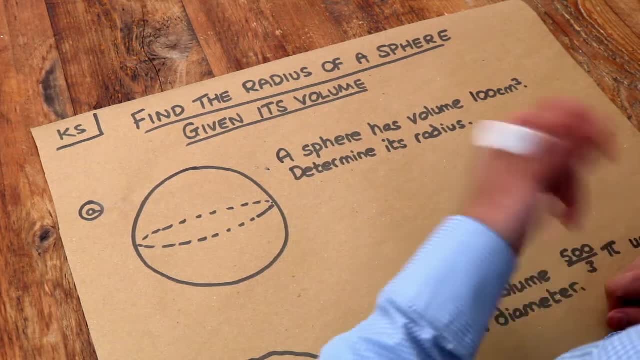 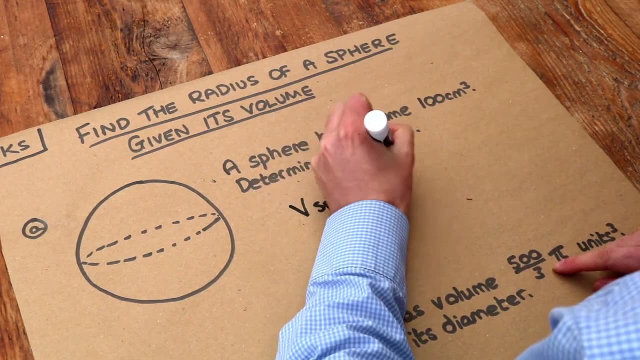 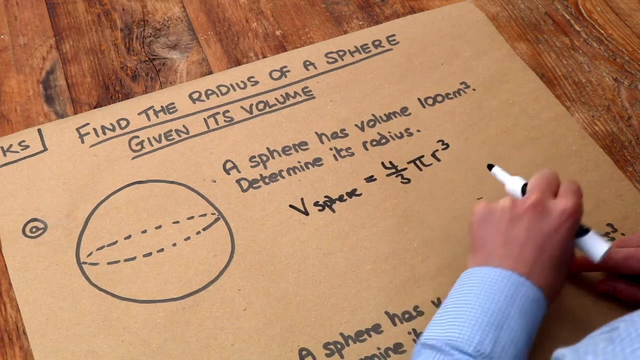 Now we're talking about the volume of a sphere here, and in the previous video we looked at what the volume of a sphere was. So it was this formula: here: The volume of a sphere is equal to four thirds pi r cubed. So that means four thirds times pi times the radius cubed. 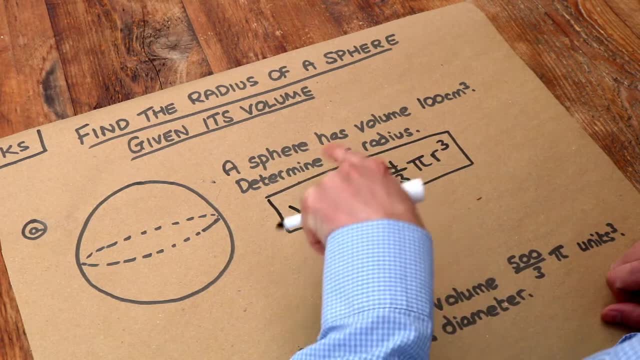 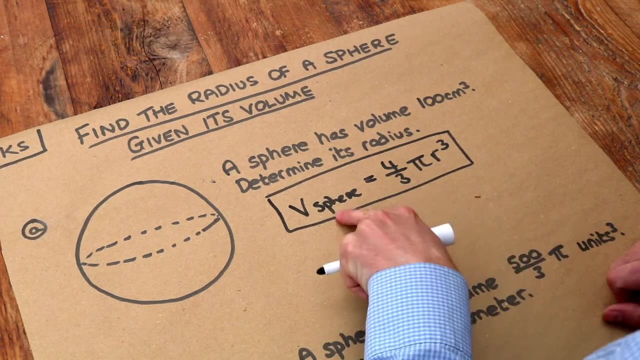 Now, before we had a radius and we worked out the volume. This time we have the volume and we want to work out the radius, But we use exactly the same method. We still just substitute into this formula. Now we're given the volume of the sphere: It's 100 centimetres cubed. 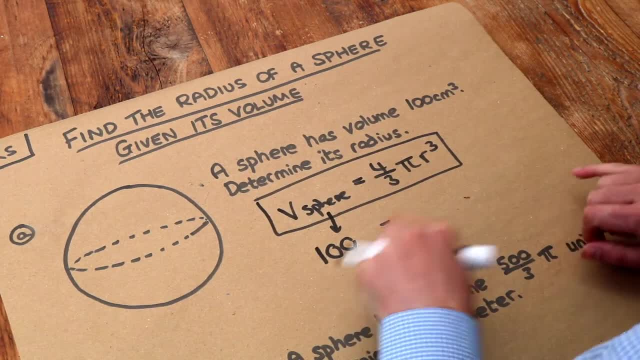 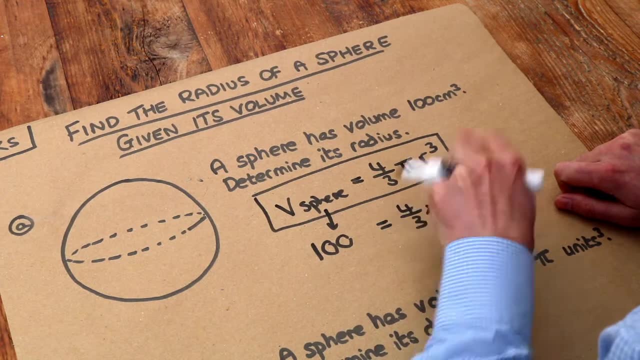 So let's put the 100 there. I tend not to put the units in when I substitute, And then we've got four thirds. That just means times by pi, and that just means times by the radius cubed. We don't know what the radius is, So let's just make it r. 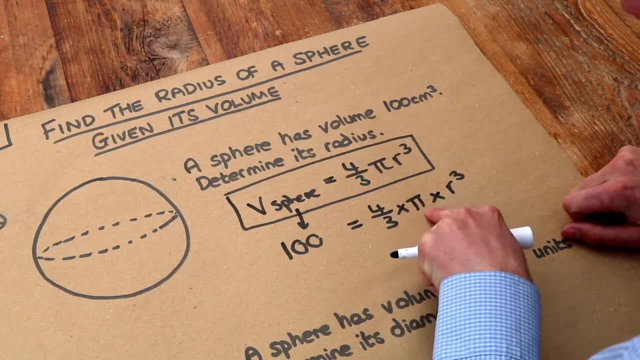 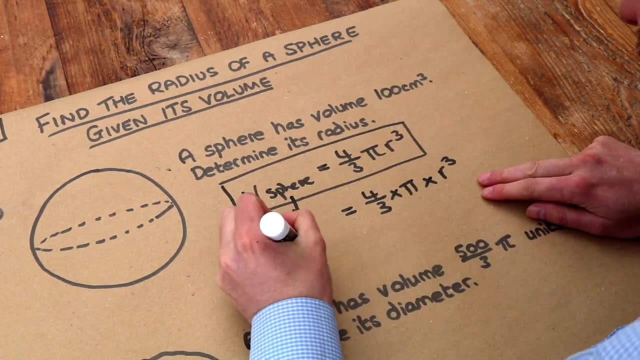 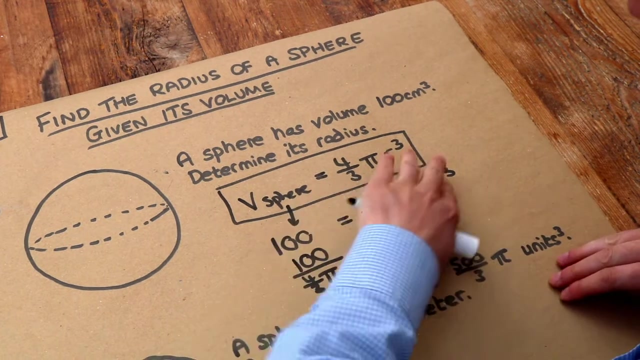 Now the r cubed has been multiplied by four thirds and pi. So we can get rid of the times by pi and the times by four thirds by dividing both sides by four thirds pi. So let's do that, We have 100 over four thirds pi equals, and then we've got rid of that four thirds pi to leave just r cubed. 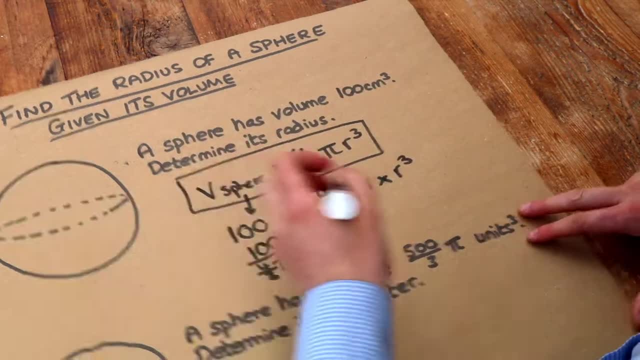 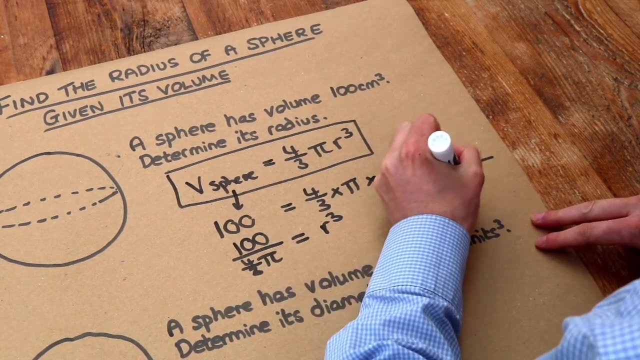 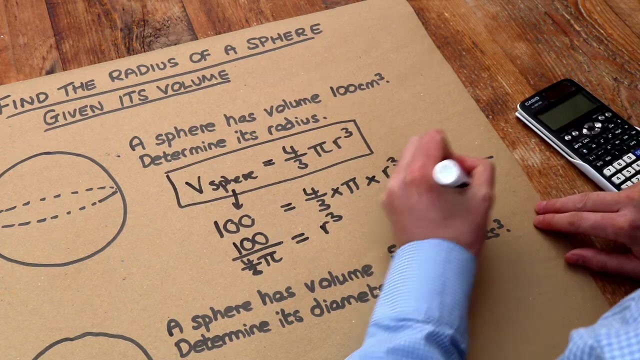 And then to get rid of that cubed we do the opposite, which is cube rooting. So r is going to be the cube root Of 100, over four thirds pi, And if you put that into your calculator you get 2.88 centimetres to three significant figures. 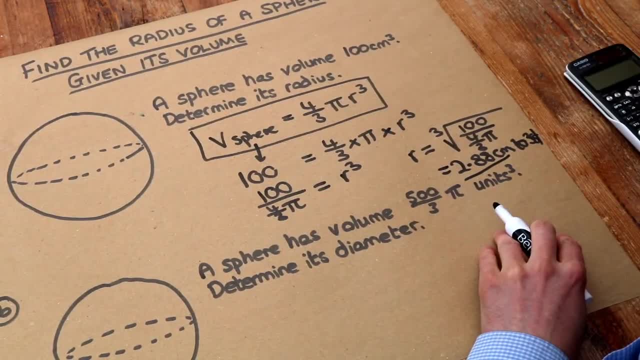 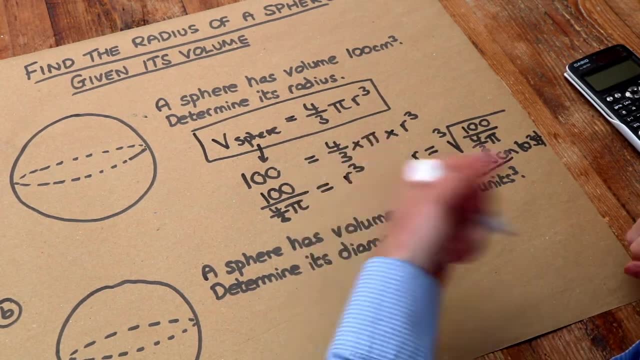 That's the final answer. What about the second one? The only difference here is that the volume is given in terms of pi. Now, when that happens, you'll typically find that the pi will cancel when you solve the equation. Let's just do the same as we did before. 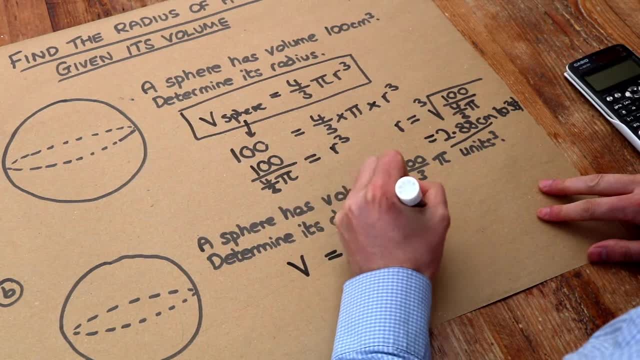 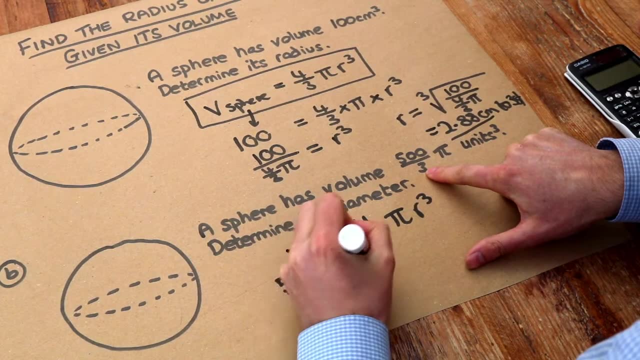 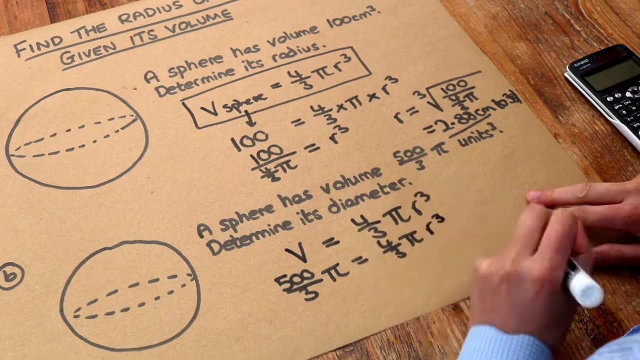 The volume of the sphere is four thirds pi r cubed. Let's substitute in Well, the volume is five hundred thirds pi, And then we've got four thirds pi times by the radius cubed. Again, let's just write r cubed, because we don't know what the radius is. 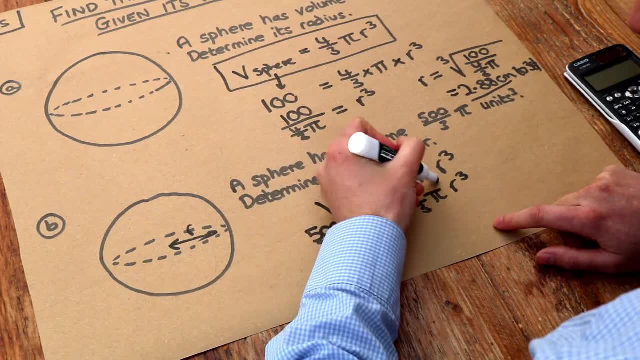 Now we could divide both sides by pi, So let's just cross out the pi's. We could also get rid of these over threes by timesing both sides of the equation by four thirds, So let's just cross out the pi's. 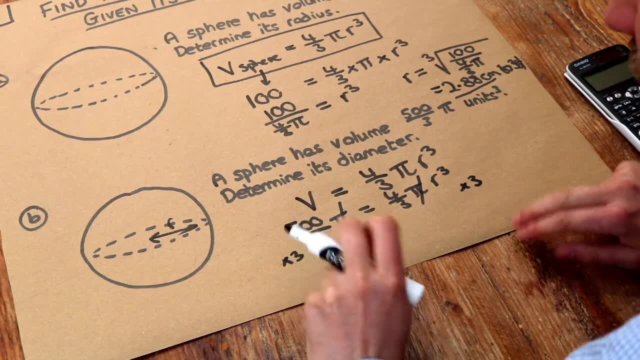 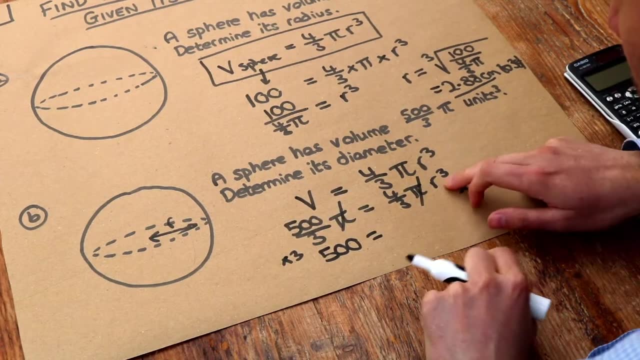 Because we don't like fractions and equations. So timesing by three gets rid of that over three, leaving just five hundred. And then the four thirds r cubed. times three just becomes four r cubed. We just times that by three to get rid of the three.